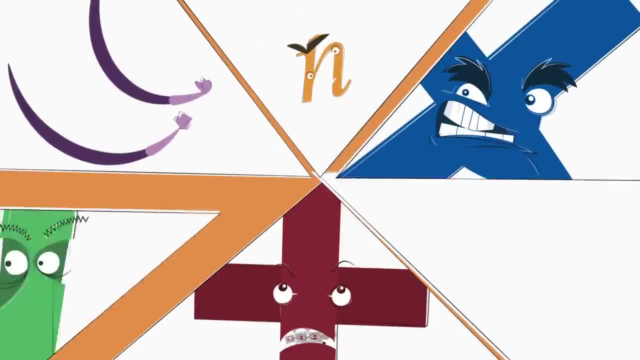 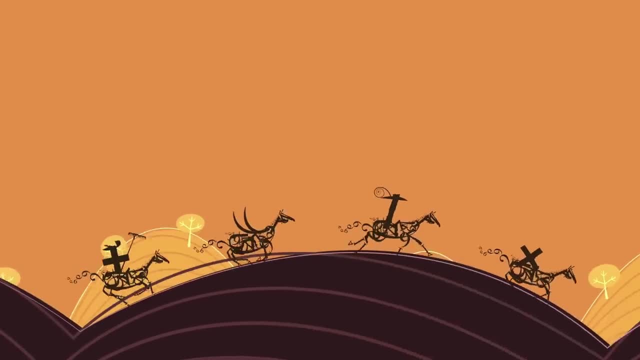 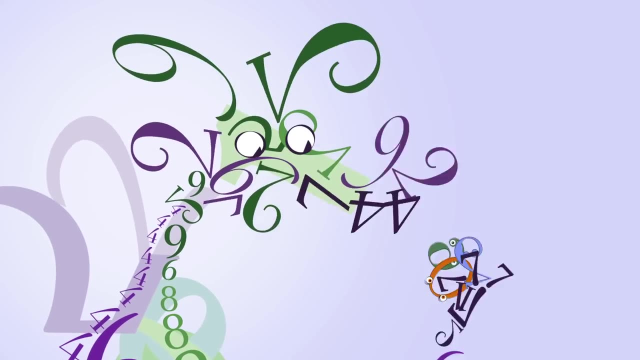 day, Anyway, the musketeers were called to action to save the land of Pi from the voracious dragon. They rode towards him on their valiant steeds and attacked: First multiplication, then parentheses. But that didn't work. The dragon continued eating people. So addition: 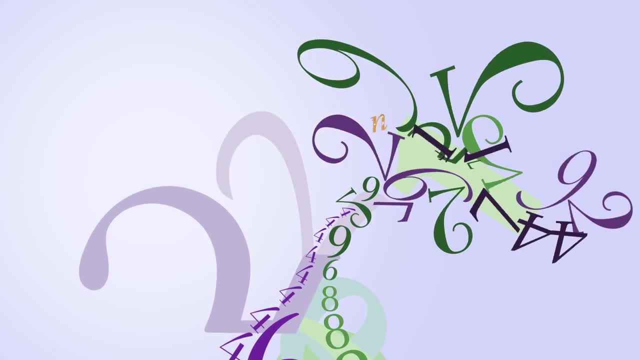 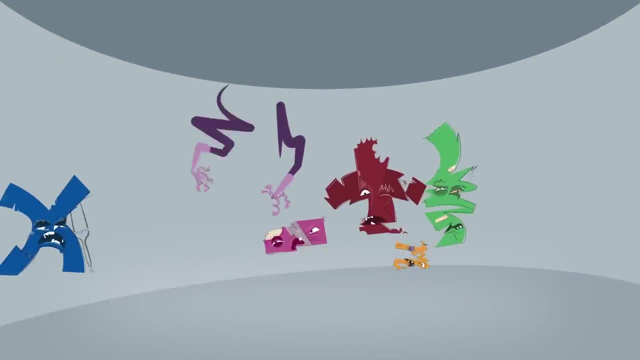 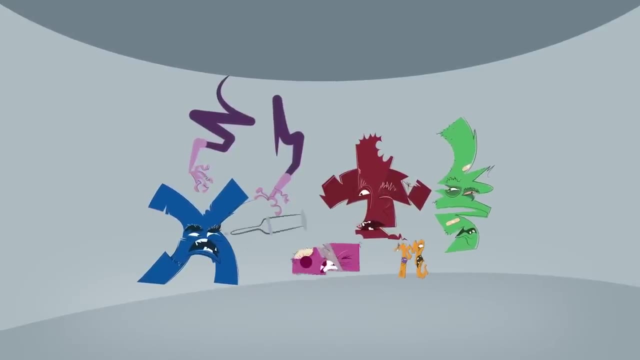 tried but was thrown aside. Exponents leaped at the beast and was quickly squashed. Nothing was working. The musketeers huddled and formulated a plan: They would attack in sequence, But who should go first? They bickered for a while. The dragon. 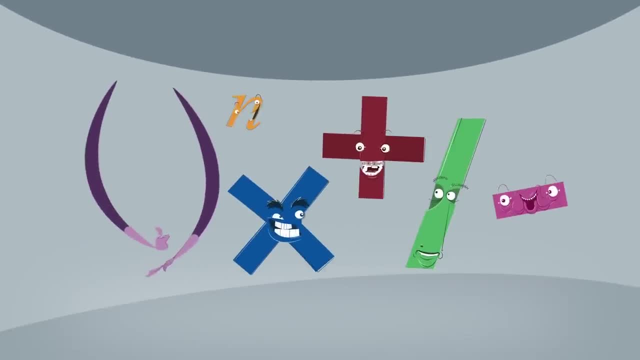 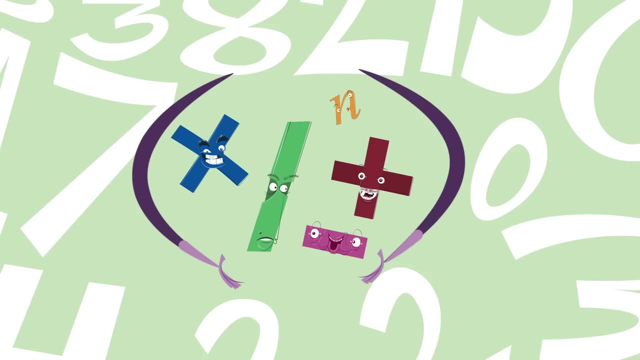 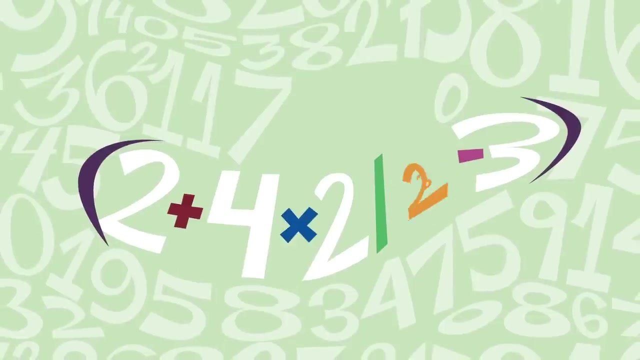 ate a few more princesses. And then they finally agreed. They jumped into the first smallest parentheses inside the great Puff. the Digit Dragon Parentheses pointed out where to work first and protected exponents, multiplication, division, addition and subtraction, while 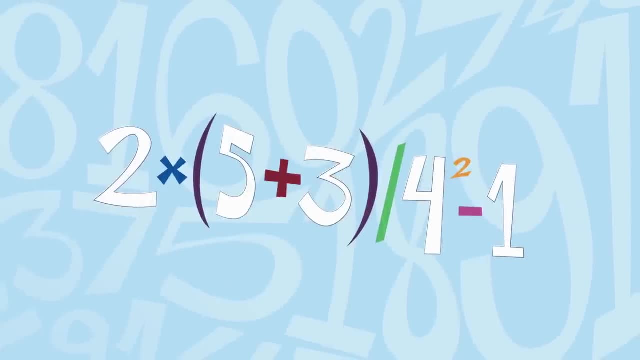 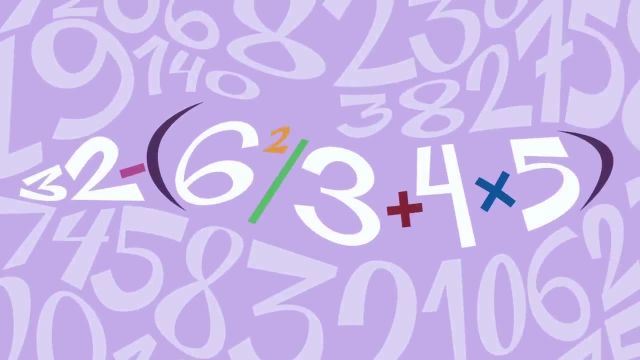 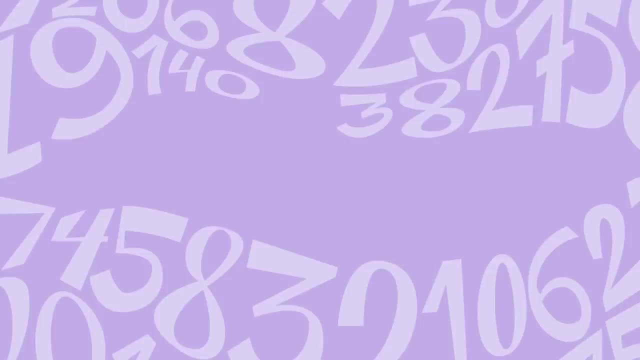 they diced and sliced: First here, Then move over there, Then there. Look out, There's another set Parentheses pointed and exponents took the lead. Then it was multiplication, division, addition and subtraction, each in turn, always the same order: P-E-M-D-A-S. When they finished, 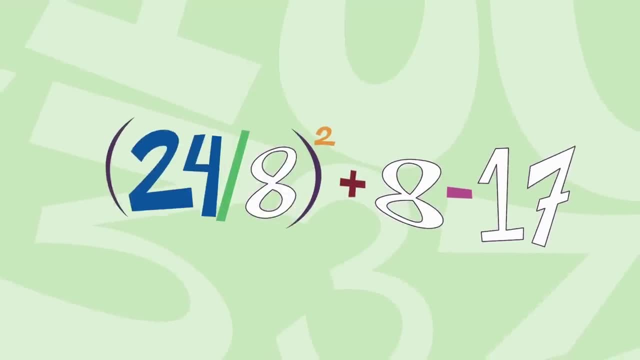 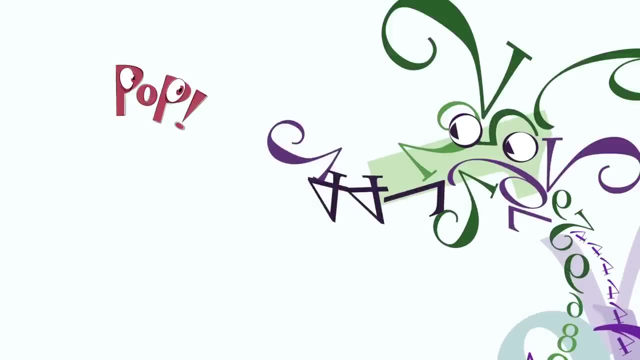 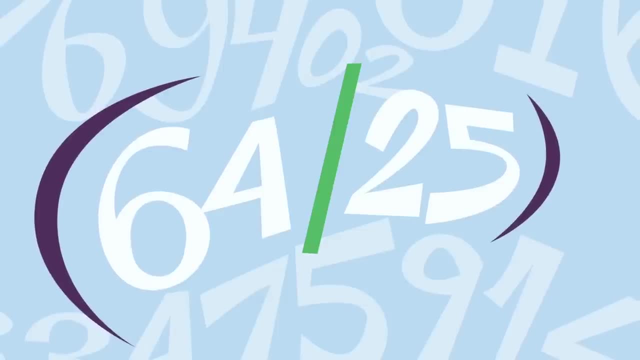 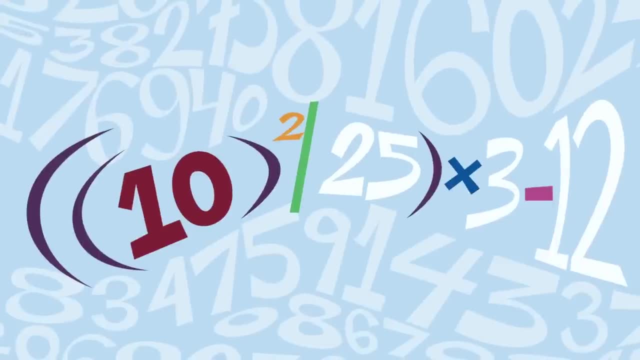 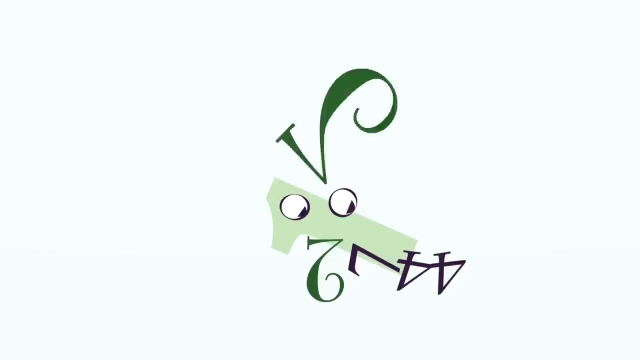 There's one And that tricky exponent, There we go, Finally. the PEMDAS musketeers had whittled Puff down to his last fearsome roar. But having vanquished Puff, the Magic Digit Dragon, all the empire's numbers sprang. 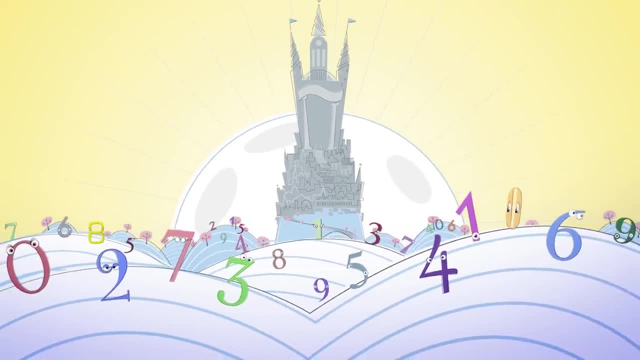 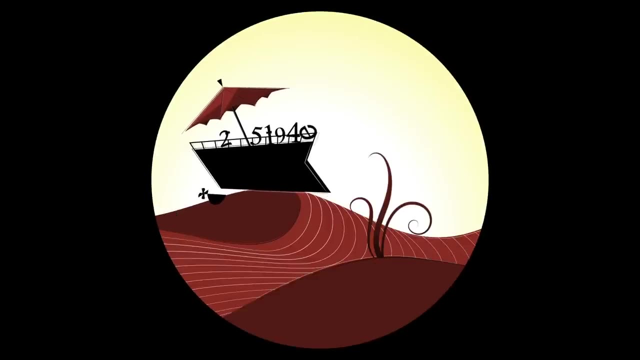 again from this tiny little number 1, and they all lived happily ever after, Except for the emperor number which they threw into the mouth of an ancient creature nesting in the desert. The end.